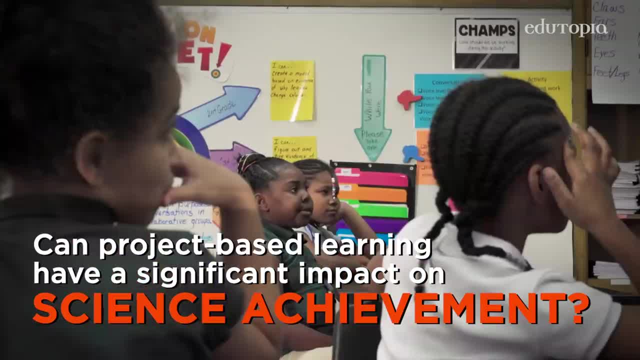 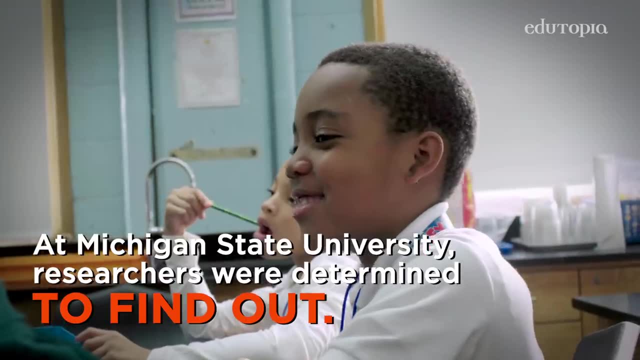 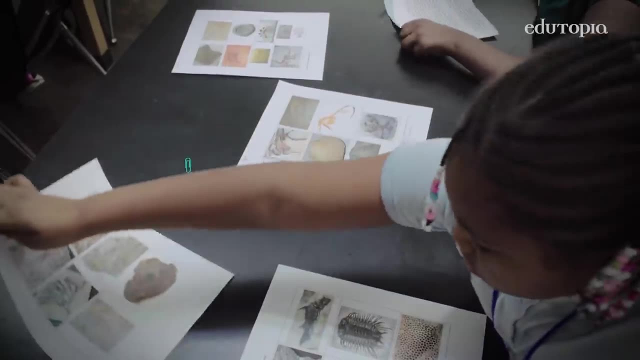 So what I'm going to do is I'm going to give you some fossils to actually look at real fossils and you can use evidence to support what you're going to tell me about the fossils. Our goal was to design, develop and test materials. The seat does project-based learning. 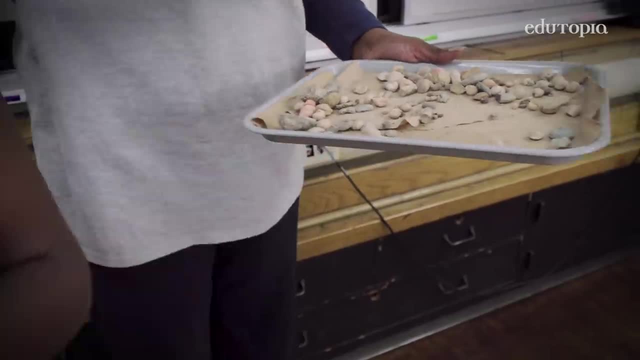 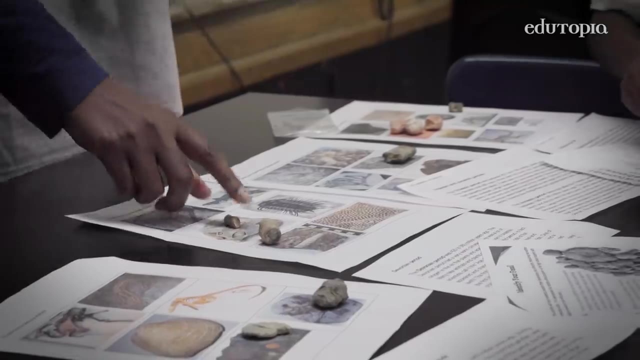 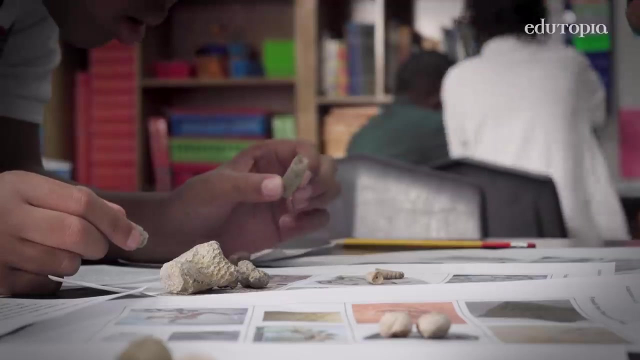 really promote student learning. All right. Kids, unfortunately, are introduced to science like it's a body of knowledge. Use your evidence to support your idea. But science is so much more than that. Science is all about trying to figure out how things work, In many respects, project-based. 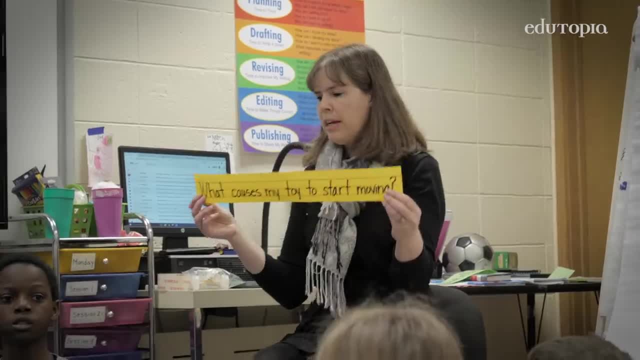 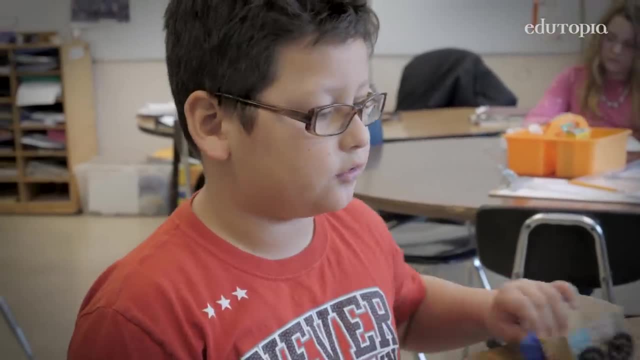 learning mirrors what scientists do right, Trying to answer a really important question or to figure out what's going on with some phenomena. When I let go, it started to go slower and slower, so then it stopped. Multiple literacies in project-based 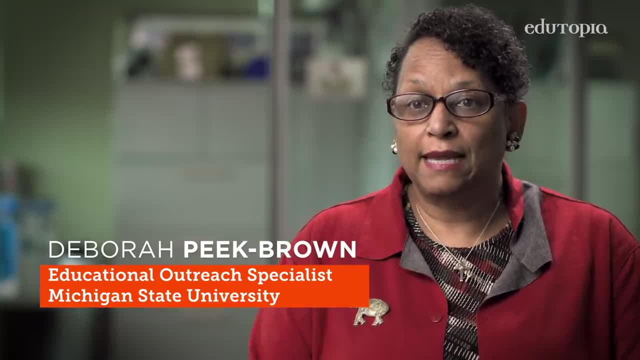 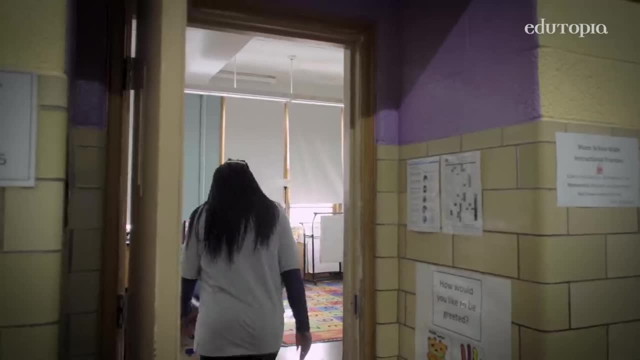 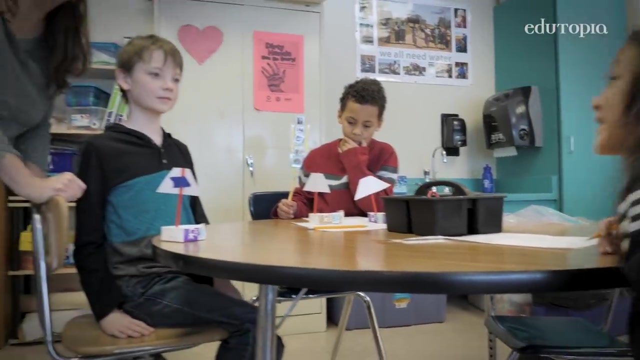 learning is very different from traditional science classrooms. I was a science teacher for about 30 years in Detroit public schools. We did cookbook experiments that usually were just validating whatever we talked about in class. When you go into a multiple literacies in project-based learning science class, you see something very different. You see kids that are 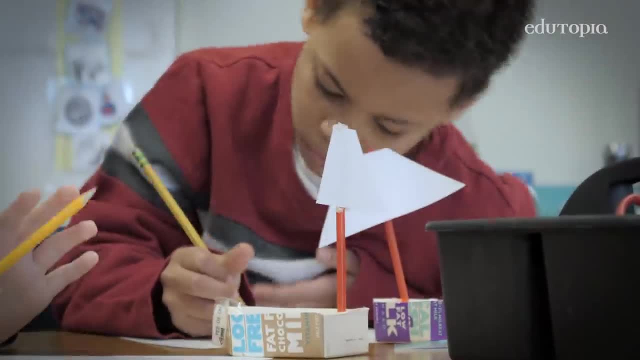 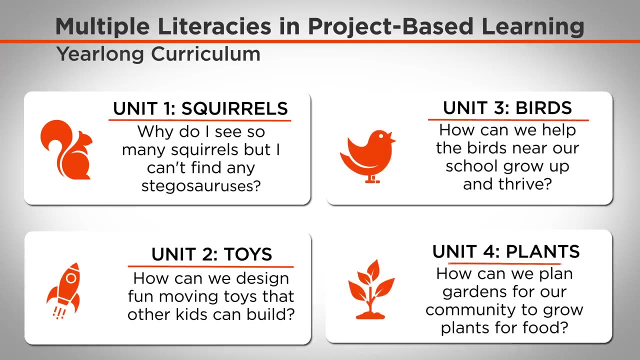 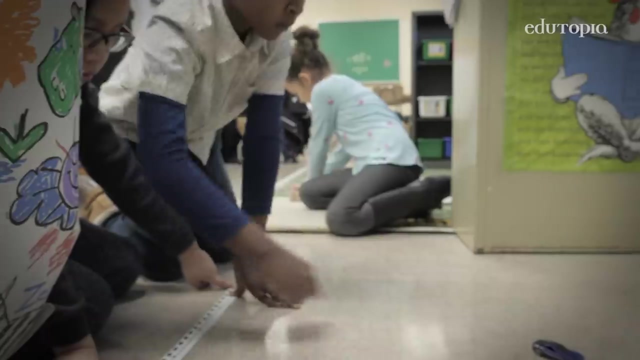 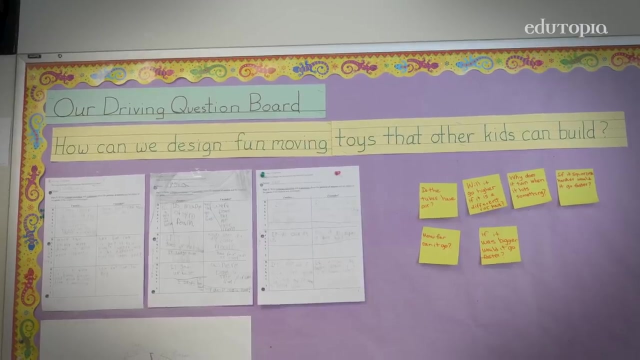 engaged in asking questions and trying to solve problems. We developed four years of units for the third grade that cover a full year of curriculum, that are integrated with mathematics and English language arts. They are really investigating things. They are really making observations, asking questions, They're developing models. They're arguing with each other about the 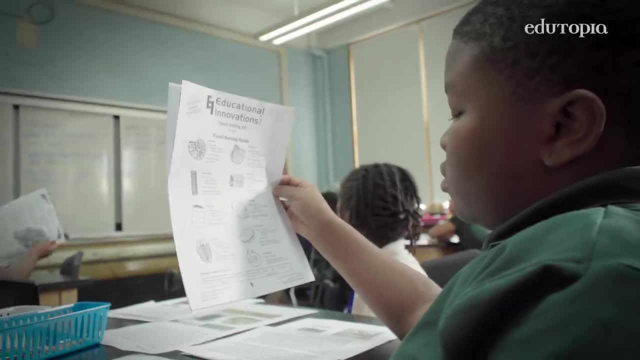 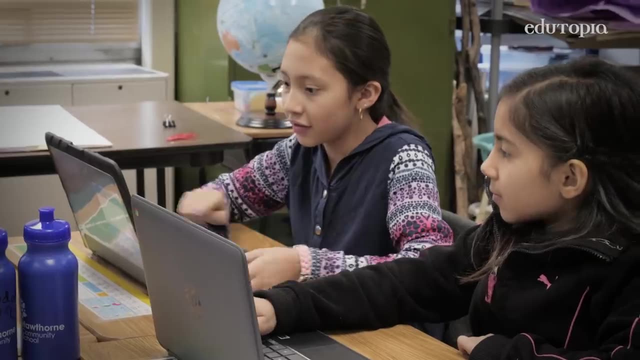 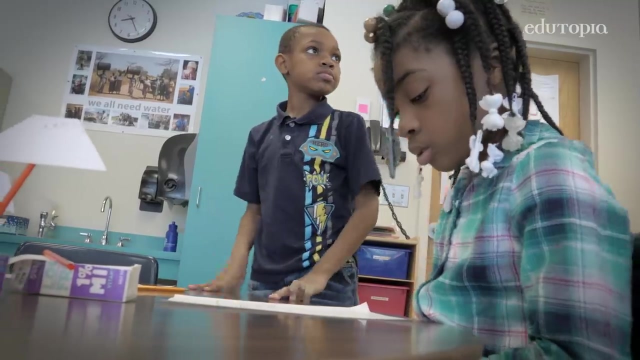 science. We integrated literacy where it was really important to support children in the learning of science. We saw just in the classroom kids getting excited about reading because they were excited about the topic, because it was something that was related to what they were trying to figure out. 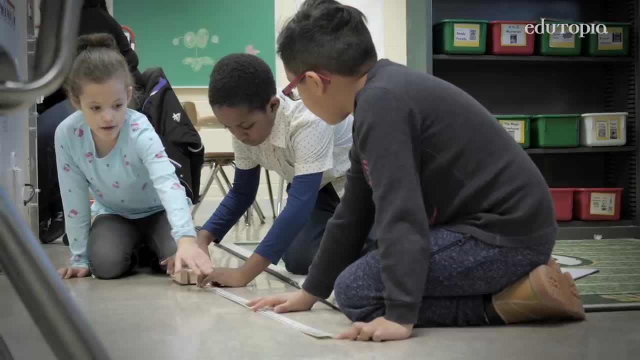 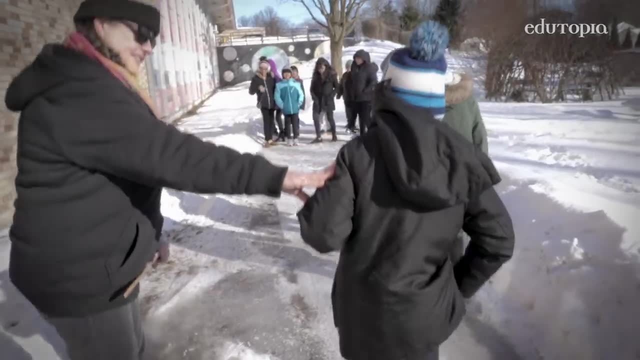 The standards in math that we chose to integrate were the ones that were so much a part of what we do in science. They were actually measuring for a purpose, in order to gather data, so that they could really analyze that data in order to figure something out. 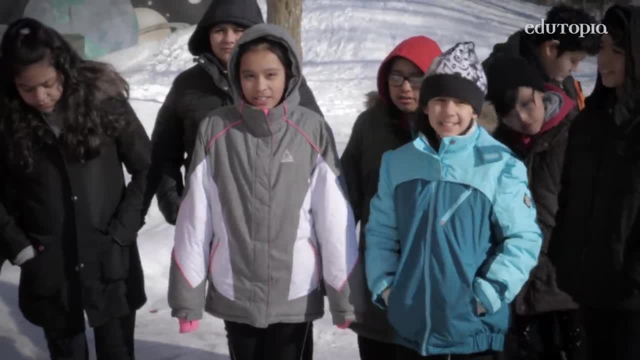 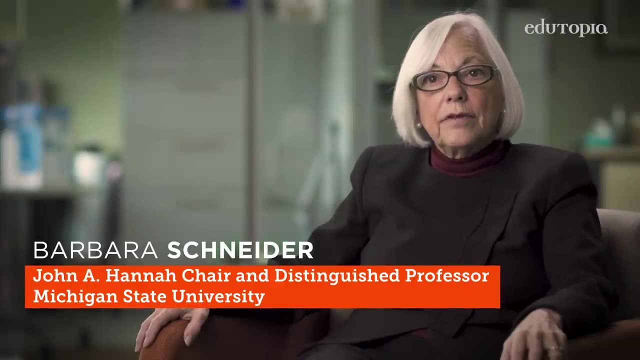 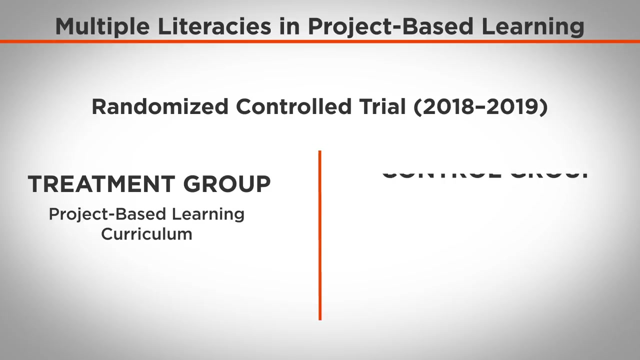 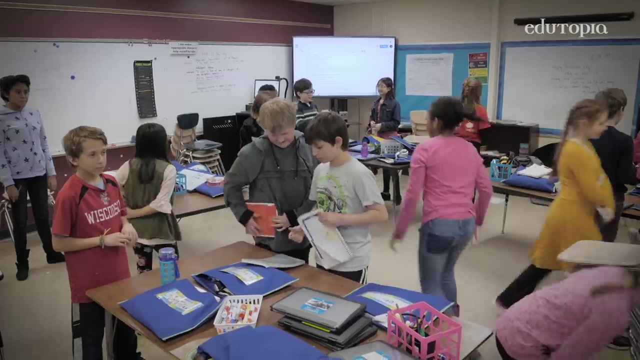 Did you see that word? No, You can't see like a paragraph out. My role in this was to help with the design of the research. Part of the group would get the project-based learning and the other group would study science just as they traditionally do. We had to make sure that our sample was balanced with 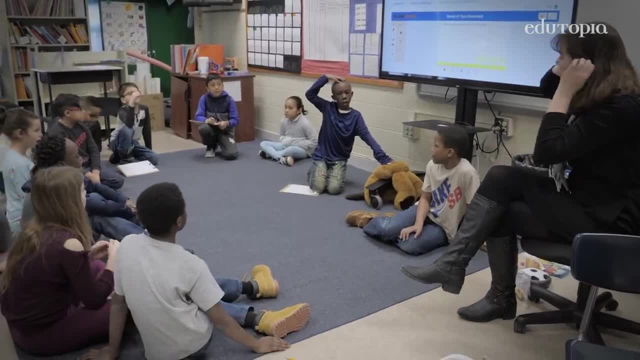 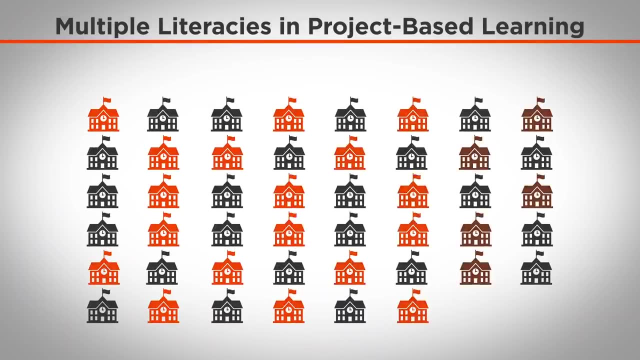 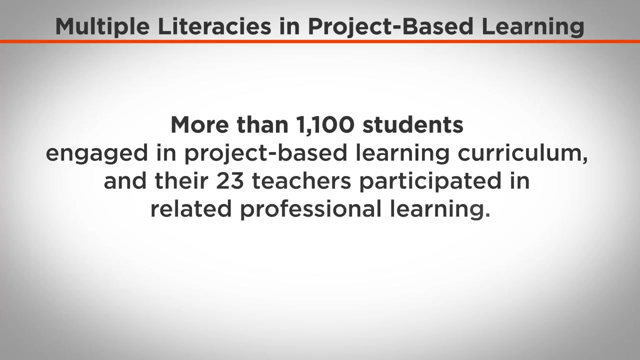 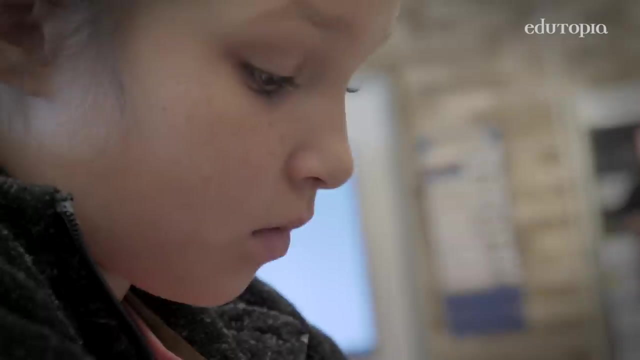 respect to their achievement, their population characteristics, school enrollment size. We looked at 46 schools: 23 in the treatment and 23 in the control group. At the end of the year we gave all the students an objective science test that was developed by the 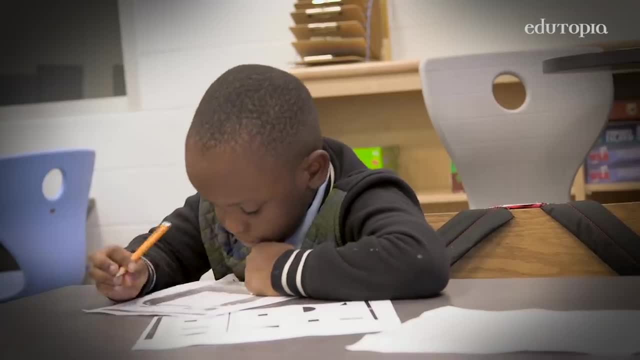 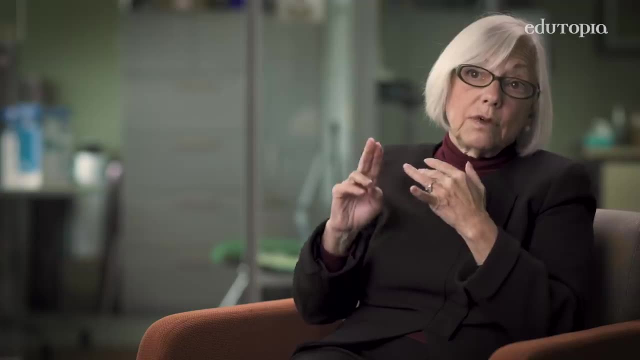 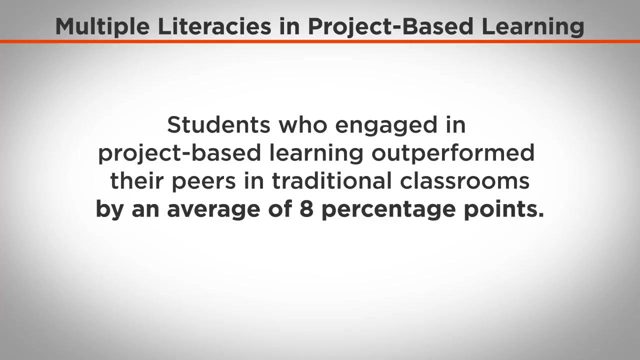 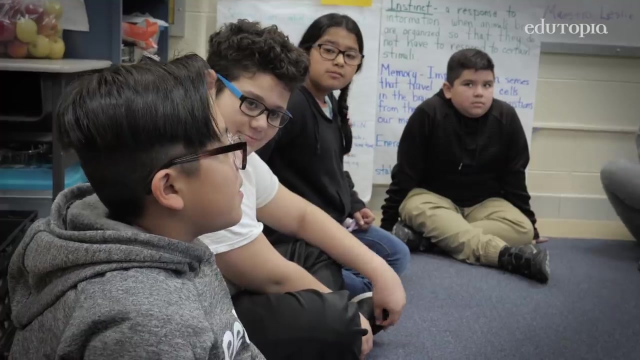 Michigan Department of Education. We found that, in fact, there was a significant treatment effect for the students that were in the treatment group. This was true regardless of what your gender was. it was true regardless of what your race and ethnicity was, and it was true whether you were a struggling reader. 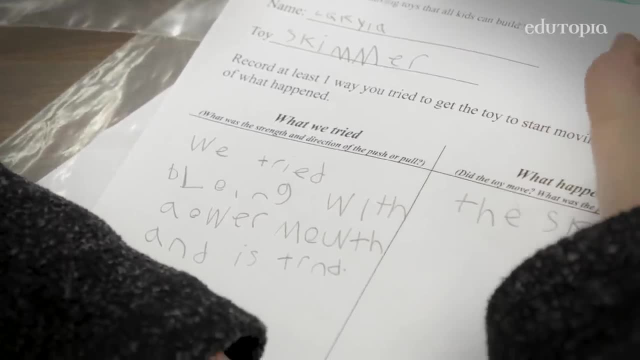 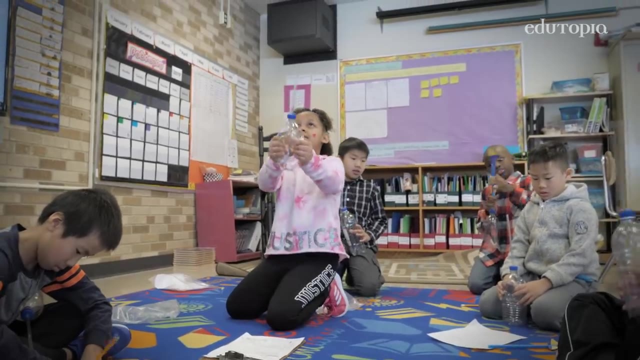 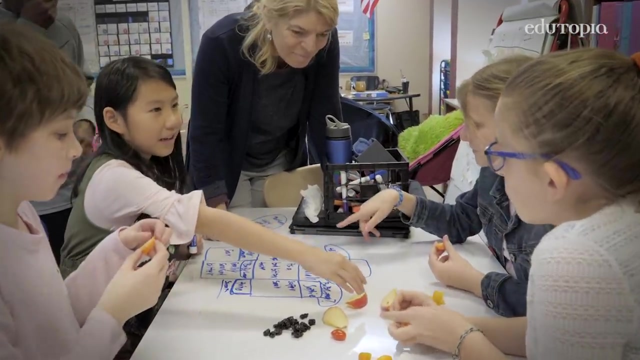 an average reader or a very good reader. We actually moved them up in their proficiencies in learning science, And so that is really strong evidence for using project-based learning in schools, because it is different, But do the kids get excited about learning science? 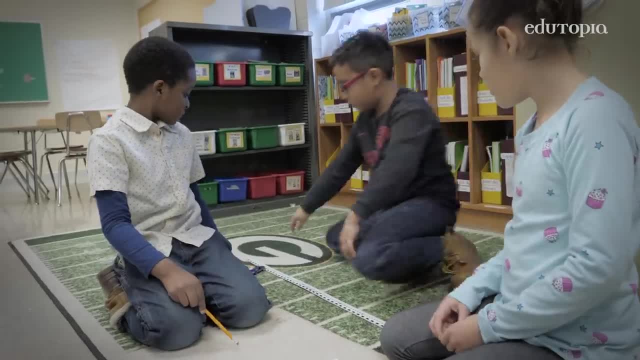 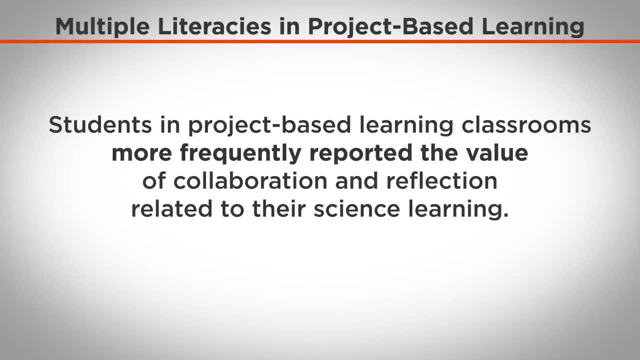 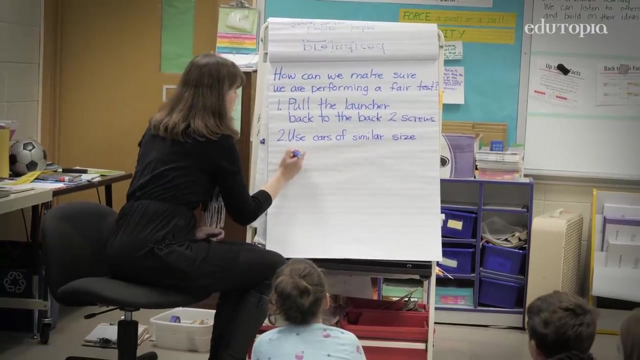 Do. they put effort into learning science, And so we also measured kids' social-emotional learning. So for teachers who are just starting out, just changing your instruction, to say we're trying to answer this question today, So so that it gives purpose to what the kids are learning. 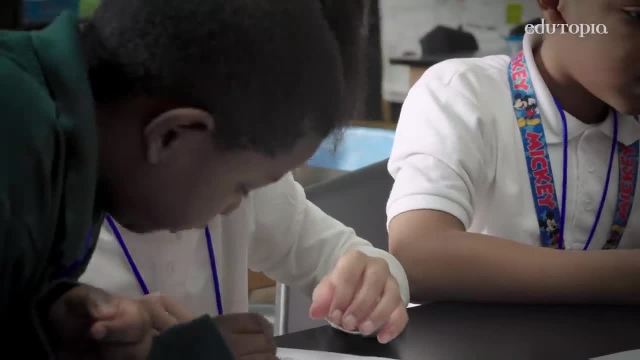 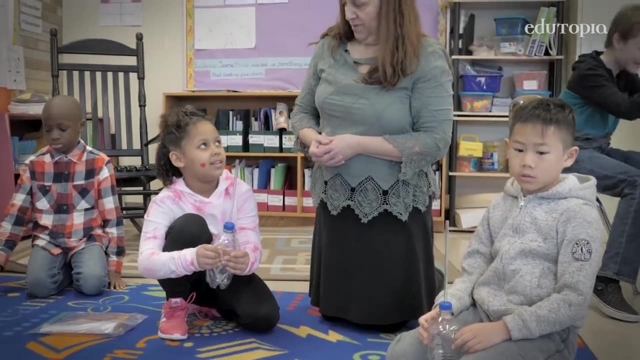 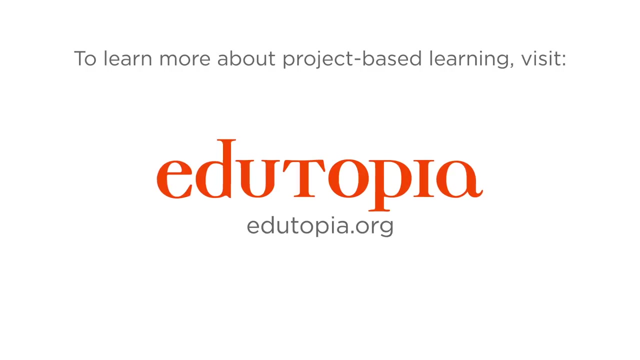 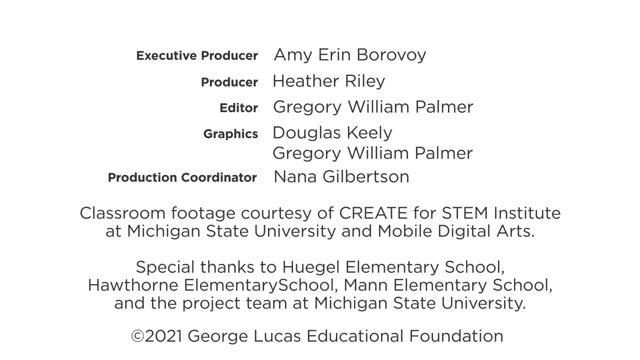 That power of I can figure things out for myself is such an important skill for kids to develop that they will be using for the rest of their lives. Did it make a difference when I changed the strap? Did it make a difference when I changed the strap? Did it make a difference when I changed the strap?